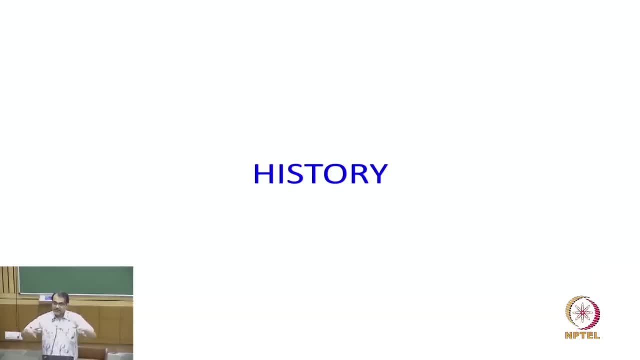 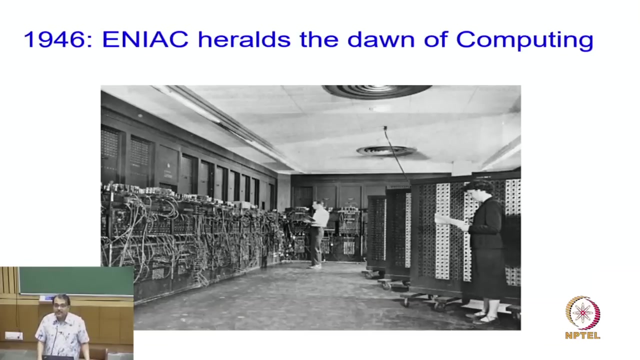 talking about the technical content. So the initial first few lectures are going to be just introducing the subject for you. And let us start from one of the salient events way back in 1940s where an ENIAC computer was constructed, designed, developed. Now ENIAC stands for Electronic Numerical Integrator. 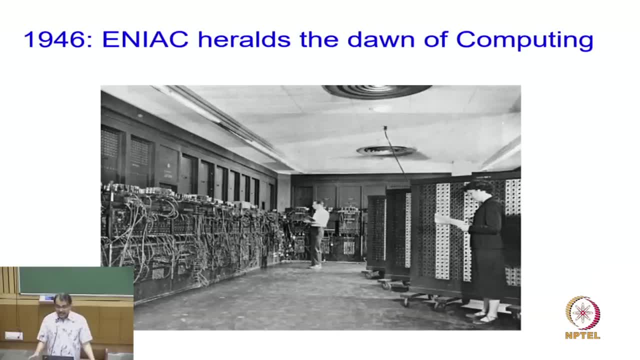 and Computer. It is the first electronic general purpose computer and it was Turing complete. Turing complete- if, for people who are advanced enough, there is a Turing machine which is the mathematical model, Okay, And it is the first electronic general purpose computer and it was Turing complete. 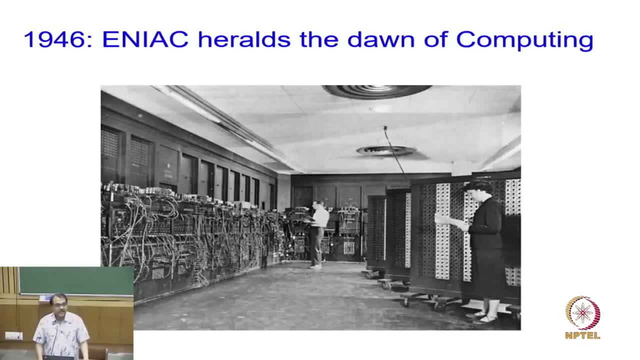 And technically, with a fixed amount of tape, the whatever Turing machine can do, ENIAC can do too, And it was capable of being reprogrammed to solve a large class of numerical problems at the time. Now let us go back to the 40s. By the way, this is one computer, just so. 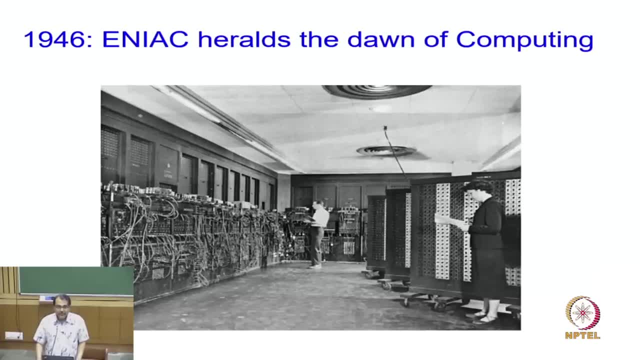 you know, And it is not. it is much worse than the computers you and I have on our phones. What would I use the computer for if I am in the 40s and I suddenly have something that can do computations? Wall supply logistics? That is a good suggestion. You require probably more algorithmics to 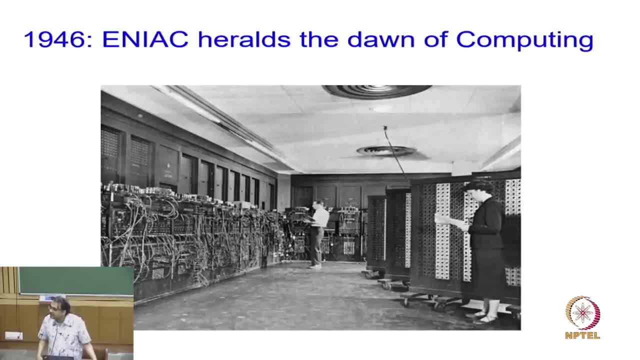 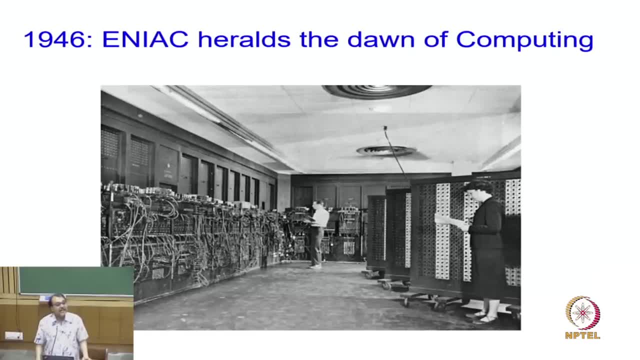 I think Alan Turing was trying some codebreaking at the time. I do not know. I do not think ENIAC itself was used for codebreaking Anybody else. So it was designed to compute artillery firing tables for the United States Army, But you. 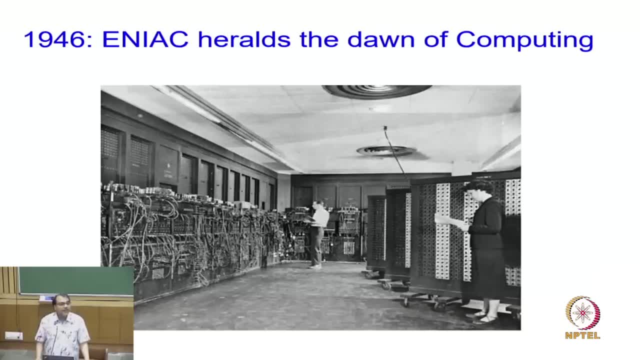 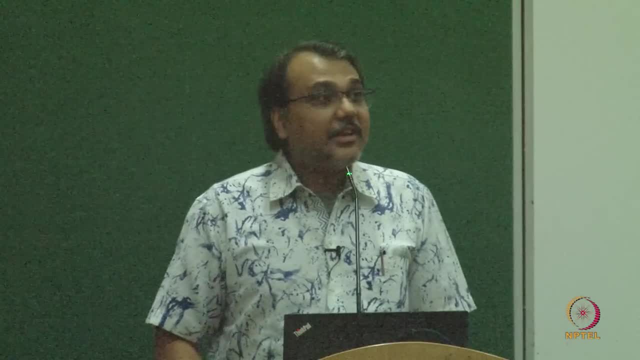 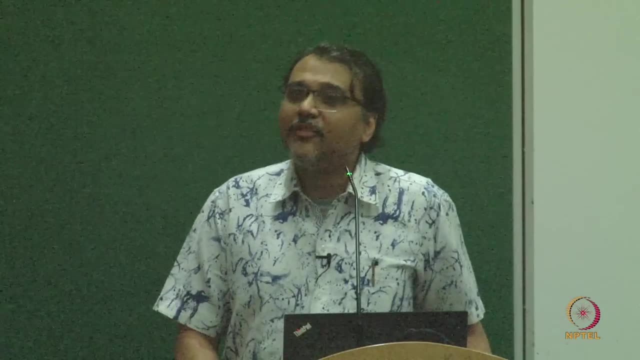 both had the right intuition in mind: It was being used for defense purposes. By the way, this is not just the 40s. I will claim that a lot of progress in AI. I will claim that that has happened because of defense and wars and enemies. This is, I mean we can smile. 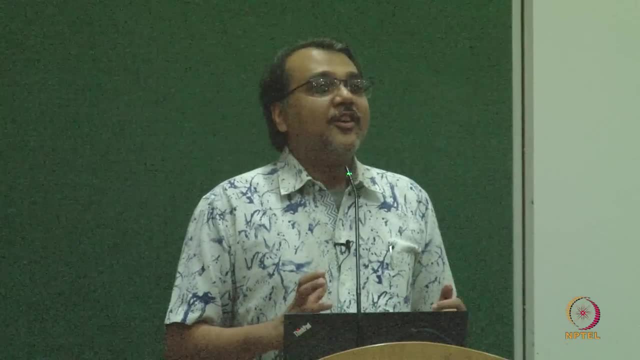 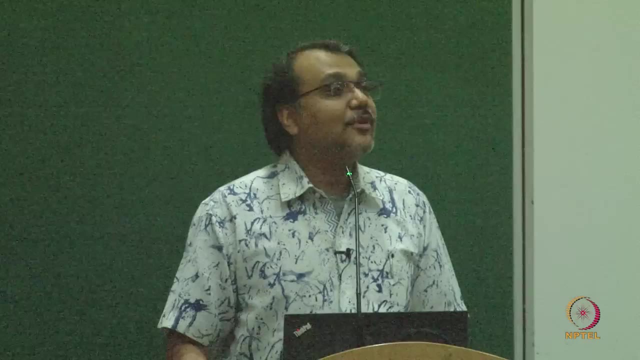 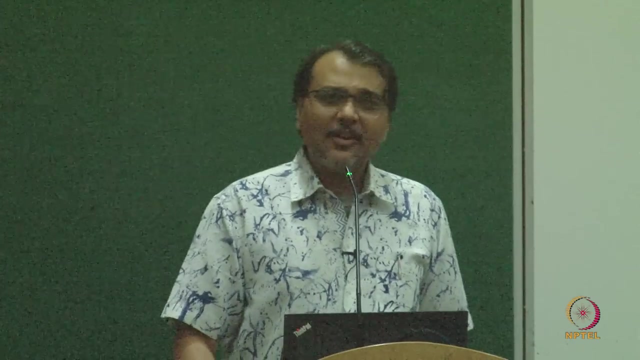 about it, but which in every country have. you see the country which puts in more money for science and less money for defense, At least some of the countries which have more money like significant amount of money. we all know US government policies. I mean they. 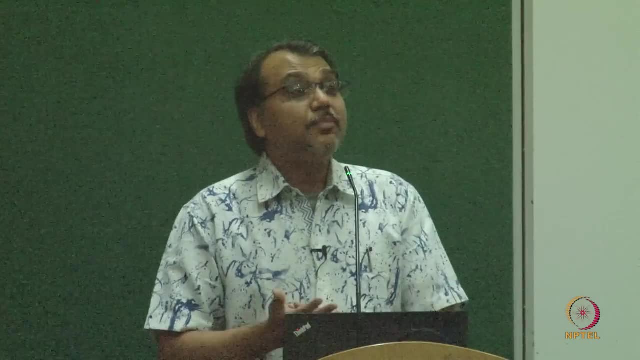 of course, put a lot of money for science, But they, I mean, are usually very specific- Yeah, yeah, you are right, You have got some technical knowledge about that, You have got. But they usually put money for science for defence or engineering for defence, right from 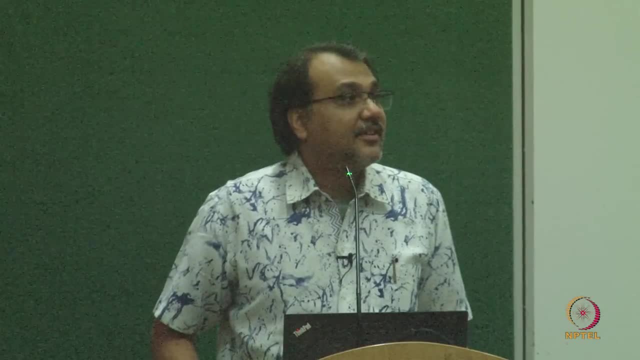 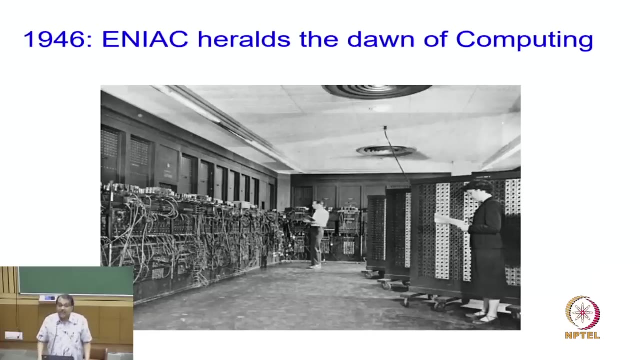 the very beginning, AI has been heavily funded by defence agencies And of course we are talking 40s World War has just happened And obviously defence is, you know, on minds of everybody. So they would create, use the, this computer for artillery firing tables. and it was said, 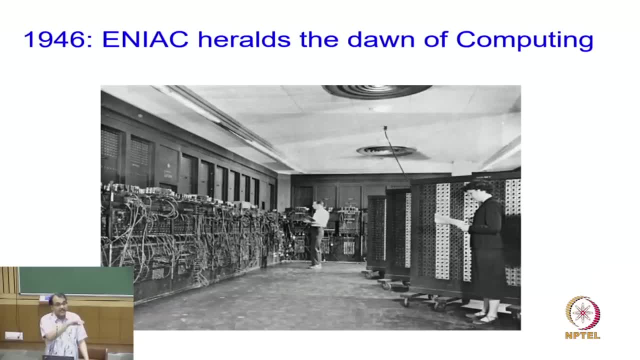 at the time that it could do things. it could compute a trajectory of a projectile in 30 seconds. where a human computer- and, by the way, we do not hear about the word human computer now. Have you heard this word human computer? You have. there was a time when there was there was a job called human computer- is a beautiful 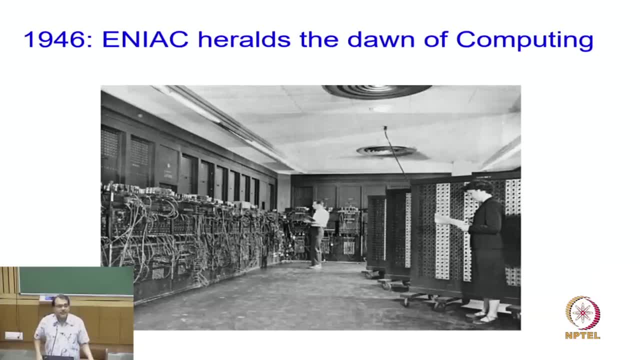 movie about NASA and three women. do somebody remember the name of the movie? Yeah, Nobody remembers. I'm sure somebody has seen it. It's about three African American women who are employed in NASA as human computers, or at least as some some form of computer. 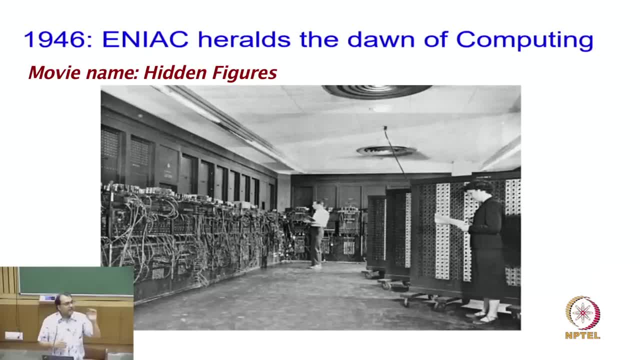 So basically their job was- and we'll find the name, If somebody remembers I can Google it, let me know. So we there. their job was to do computation And they would compute the these projectiles, And they may take about 10 hours to compute one projectile trajectory. 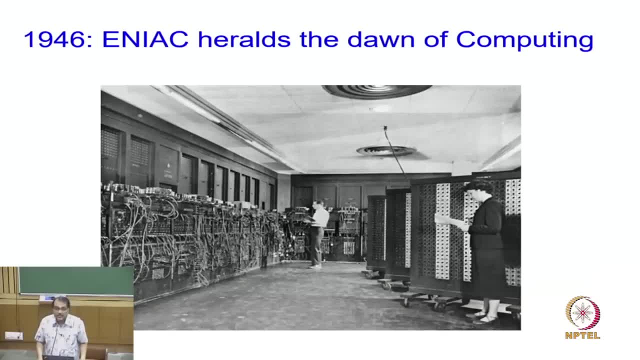 And this thing can do. the ENIAC could do the same thing in 10 seconds, 30 seconds, right. So notice that right from there. and of course now human computers is not a job Not surprising. There is also a beautiful story about a woman who really got a bunch of these women together. 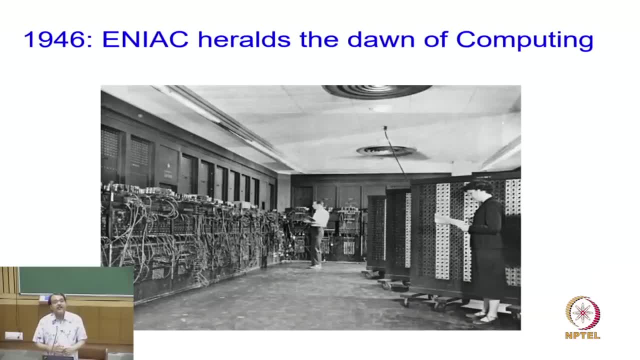 and train them as human computers in a time where these women did not have a computer. So this is a beautiful story about a woman who really got a bunch of these women together and trained them as human computers in a time where these women did not have a computer. 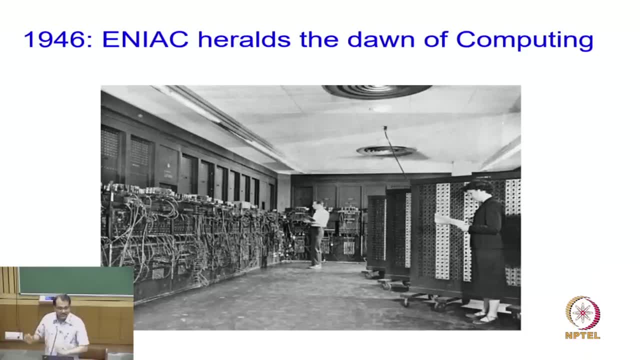 Okay, You know, they have much to eat and so on. That's a different beautiful book, But anyway. so that was then right. And now that this was the time and computers were coming into the fore, right. It was a reality, not just a figment of somebody's imagination. 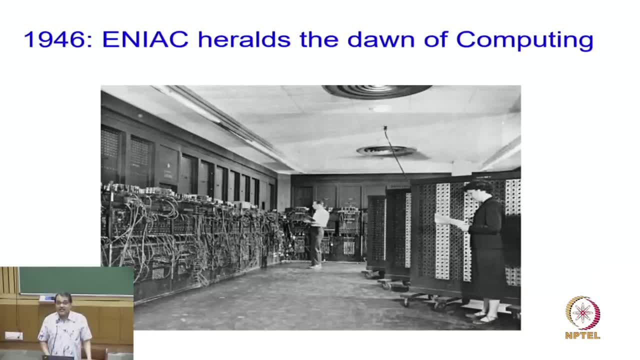 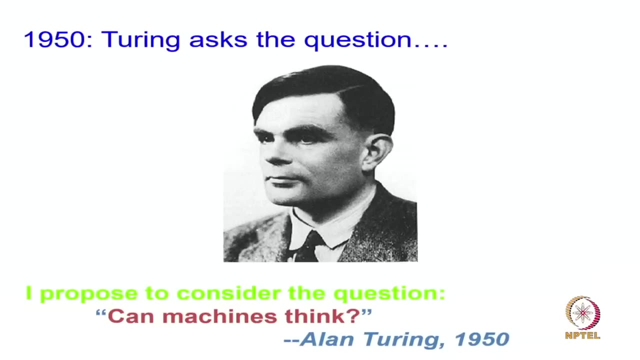 They did not ask the question: can I use computers for word processing Or can I use computers for Excel, like spreadsheet management, All maintaining my database? In 1950, Alan Turing, who is considered the father of computer science. You all know about Alan Turing, right. 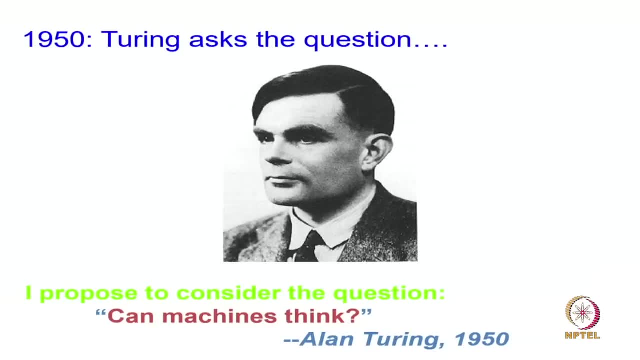 Some of you may have seen the imitation game. Yeah, You must see that movie, beautiful movie. He said in his seminal paper that I propose to consider the question: can machines think? That is why we call him the father, Because that particular question that he asked in 1950, when this one big computer or you, 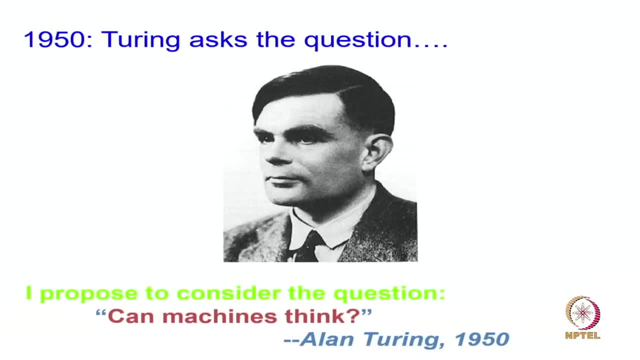 know, some of these computers have just started coming out and the only thing they are doing is computing the trajectory of projectiles and so on, so forth. He is starting to think as far into the future as possible and being somewhat of a luminary and writing these seminal papers, thinking about these philosophical questions. 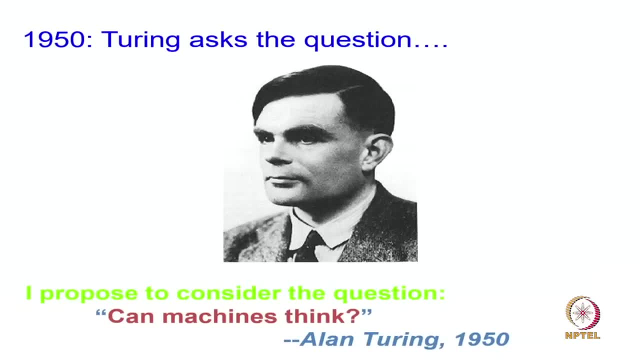 And he asked the question that okay, let us say a machine can think. How would I know that it thinks? Now think about this question for a minute. Suppose I claim that this podium, which is made of wood, thinks, has the ability to think. 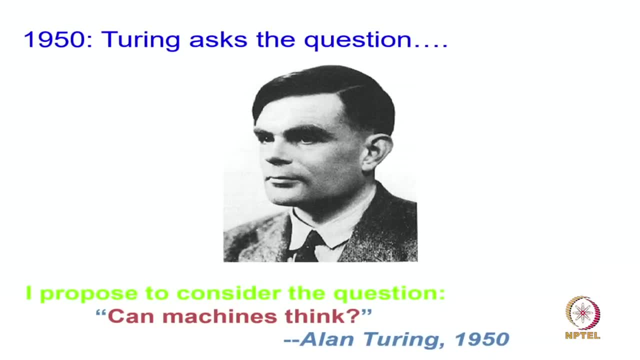 without casting any judgment on what wood is made of, and as I mean what, what is wood? and whether we have any prior on whether this is living or not living. let us not worry about this. Let us say- I make this claim- that this podium thinks. 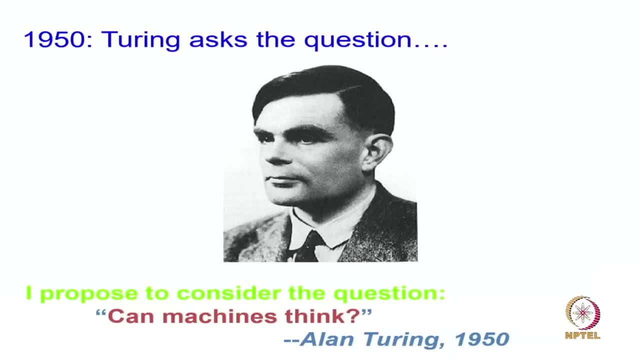 How would you and I even assess Whether this podium thinks or not? Now let us take another example. Whenever we ask such philosophical questions in AI, we relate them back to our life. Suppose I have to ask the question: does my friend think? 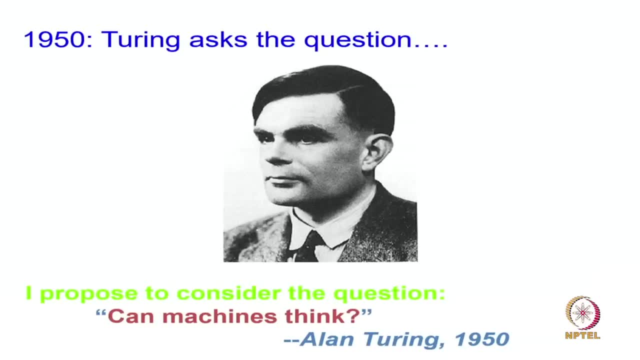 What would I do? I would ask them a question. I would ask them a question which I think my friend should give a correct answer for. Okay, What would I want to believe that this person really thinks Right? This is a good question. 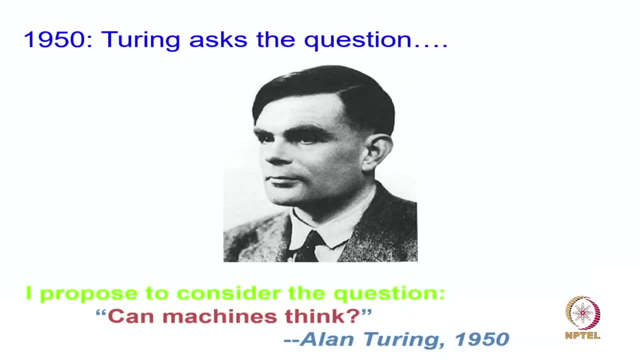 It is an intelligent question. If I ask an intelligent question and my friend is able to give me an answer, then I would make the claim that this my friend thinks. Suppose my friend could not speak, What would you do? Written answer. Suppose my friend did not have any hands: 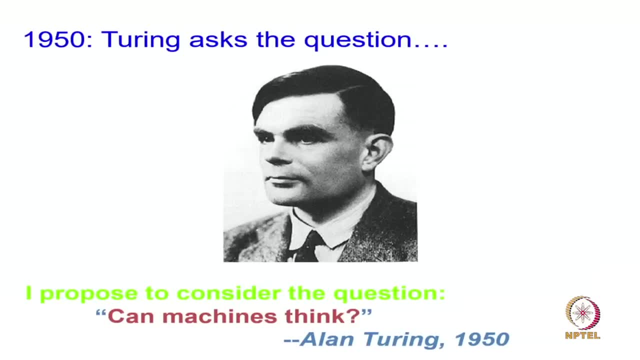 Sorry, Another person could write for them. Another person could write for them How, If they do not have hands, create a situation that they have to make a decision, and decision would be seen by some movement of hand, blinking of eye, you know, movement of arm moving. 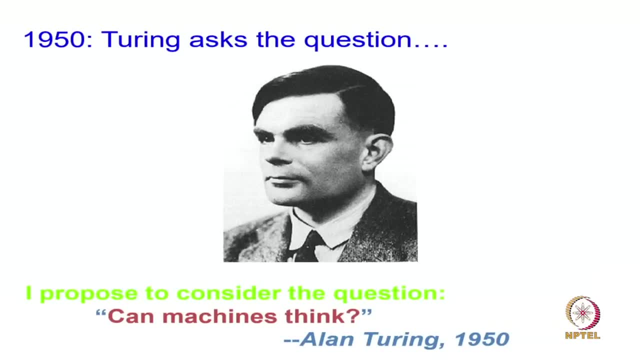 of legs, whatever right Suppose they did not even have an ear and an eye. Now I know why we do not want to visualize such a person, and it is becoming very gloomy at this point. But think of it as a thought experience. 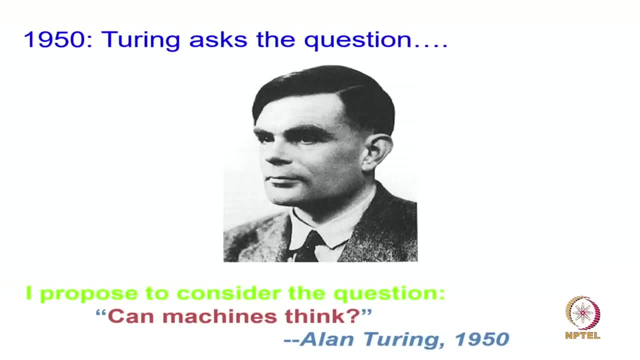 This is probably what Alan Turing also thought about at the time. I do not know. Hopefully, Suppose I have a person who cannot see, who cannot observe the environment, who cannot make a difference to the environment, does not have hands, does not have voice, does? 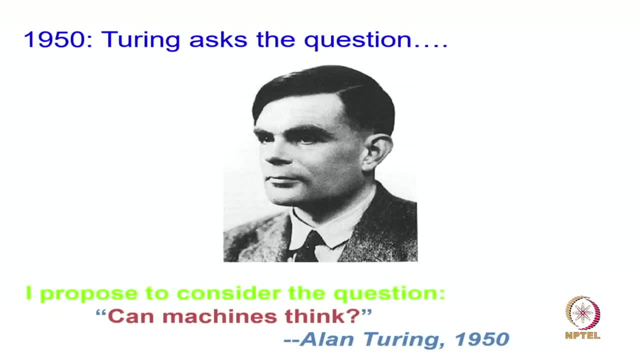 not have eyes to blink, does not have any motors, has a brain inside. Is it possible that this friend, this person, not friend- does not have eyes to blink, does not have eyes to blink. This person still thinks, but we will have no idea about it. 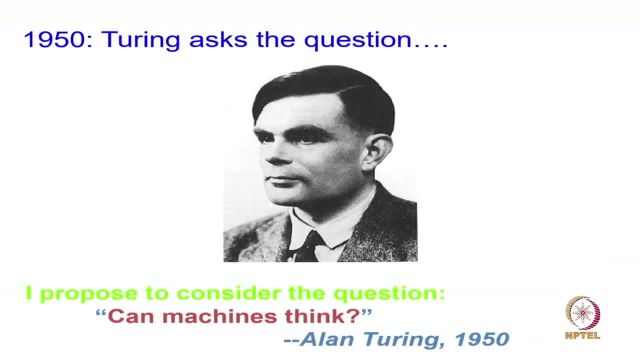 Is it possible, Come on, at least nod one way or the other. Yes, it is quite possible that, and you may have seen, and sometimes I met a person you know who had Parkinson's disease, but the Parkinson's disease had, you know, gone to. 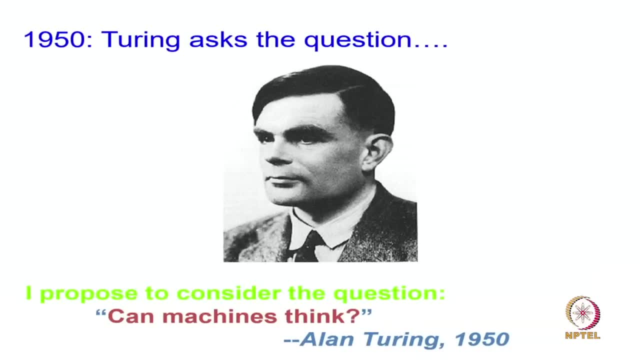 a certain extent, that there was full paralysis and so the person was not able to communicate very much, and we did not know very well whether the person is able to observe the discussion or not, whether the person is able to understand what is going on around their surroundings. 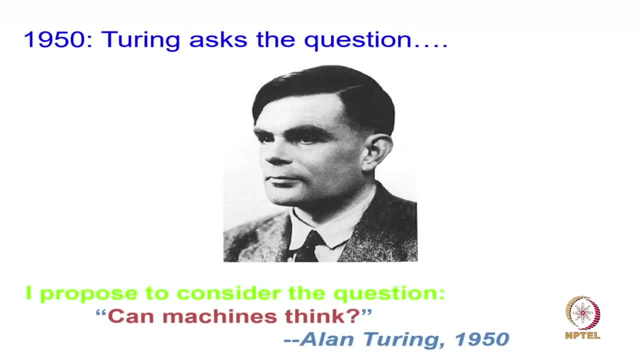 or not, This is even possible in a human in today's world. It is possible that their brain was working perfectly. They just had no way to communicate. It is possible that their brain was not working at all and we just have no idea. 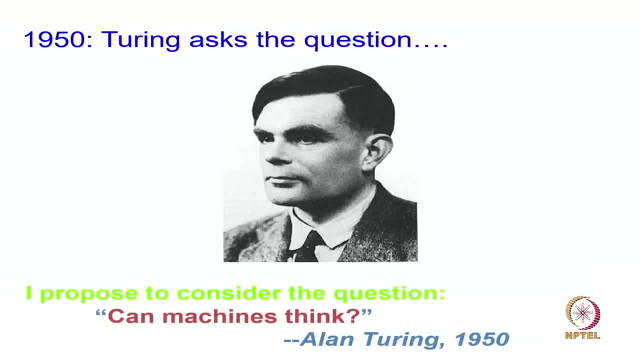 So the point is not working at all means. not working internally, Yes, In terms of the what understanding perception of the environment. So the point that Alan Turing came back with is that it is possible that this podium thinks we have no way to know because the podium has no way to communicate with us. 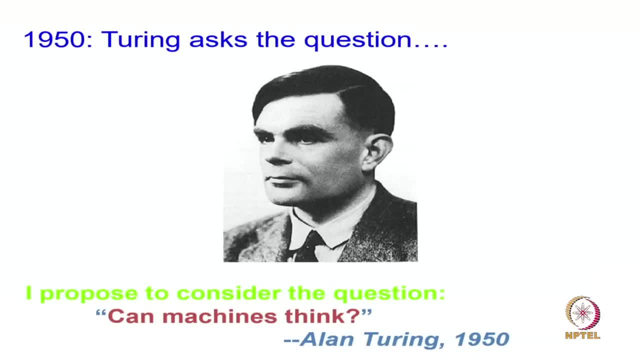 So you will, over time, see that communication with the world by listening, producing an output- not listening by ear, necessarily by observing, or by looking at the environment, perceiving the environment and then come out producing an output- is critically important for us to judge whether there is an AI system sitting in there or not. 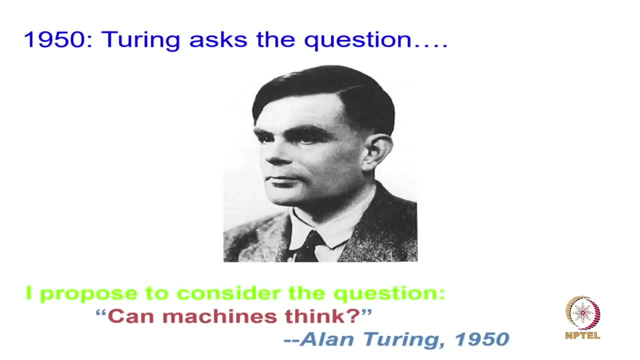 Because the brain is meaningless in absence of the communicators in the body, And therefore he said that the only way we can figure out that a machine thinks is by asking it questions or creating a scenario where we can judge its decisions, And he devised the very famous Turing test. 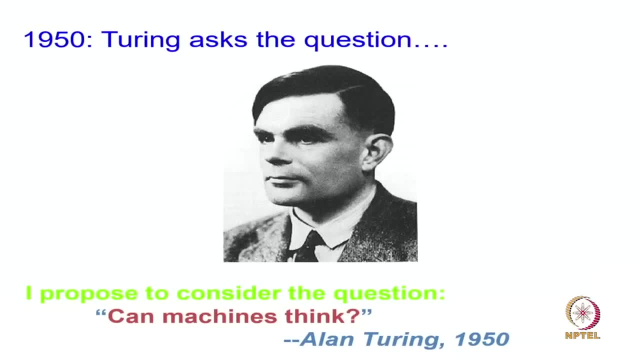 I am happy Many of you know about it. It has become part of a you know folklore of AI and folklore of computer science And we will talk more about it at the time a little later. But he said that the Turing test would be a good test to figure out whether machine 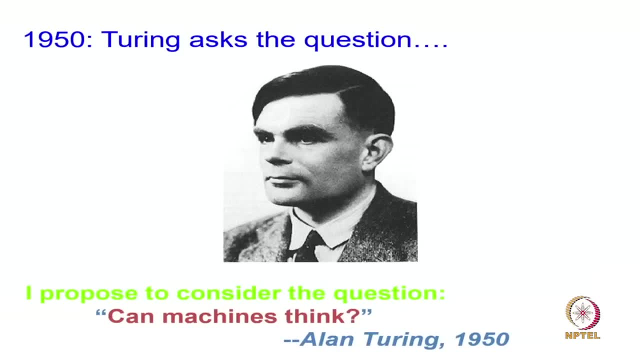 thinks or not Notice. by that time, the field of AI is still not born. This is still his thought experiment, and he has written this paper. Now, of course, this idea starts to pick up And in 1956, four of these people come together. 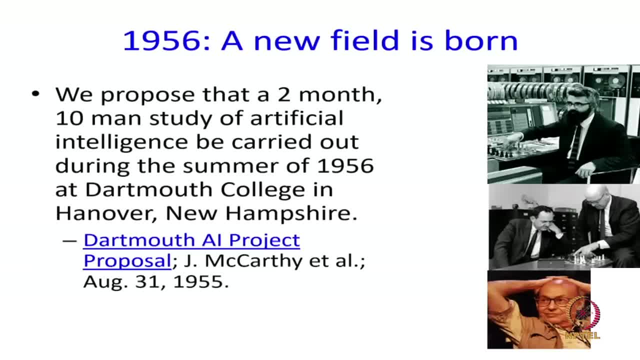 Yes, They come together to do a two month workshop at the Dartmouth College in 1956. These four people are called the founding fathers of artificial intelligence. They say in their project proposal: we propose a two month 10 man study of artificial intelligence. 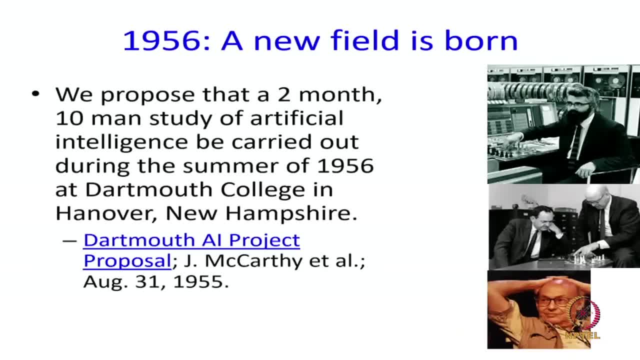 This is the first time the word artificial intelligence starts to get used, And it was given by the very first person on the right, John McCarthy. Now, John was at Stanford, He worked a lot on chess And he also created or co-created the language called Lisp, which is a declarative programming. 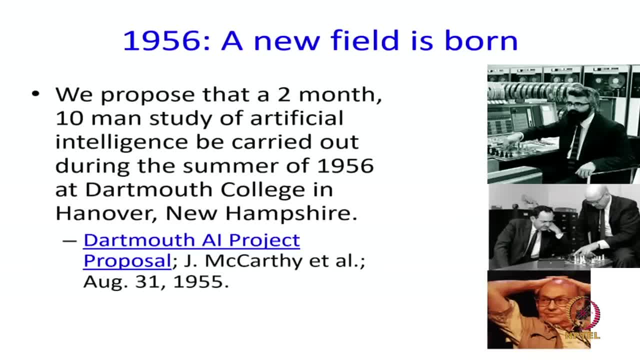 language which became very popular in the 70s and 60s. They say that in two months we will solve artificial intelligence, And they meet together at Dartmouth College over the summer And that is where the field of AI starts And that is where the field was officially born. 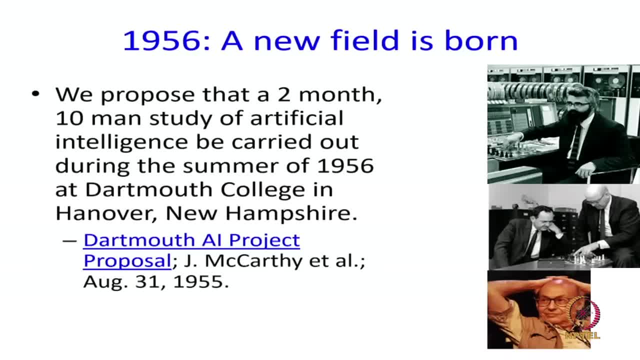 Of course, they had to spend more than two months for AI to be solved, and we have still not solved it. So, therefore, there is one thing that I feel when I think about most AI researchers is that they are highly optimists, heavy optimists. 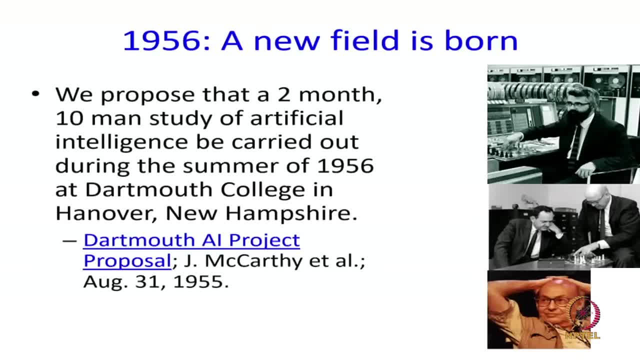 They feel that we can do something much before anybody in the world is ready to achieve it. And they of course fail, but that is okay. They move the field forward, And these were the four optimists who thought that they can solve most of AI in two months. 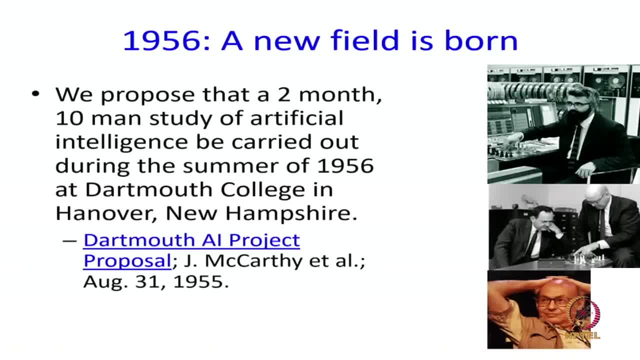 This joke, but that is somewhat true. also. Let us talk about the other three people. Alan Newell and Herbert Simon are in the middle. They were from CMU. They were working on logic theorists. They were trying to figure out: can we somehow create a theory of how to prove theorems? 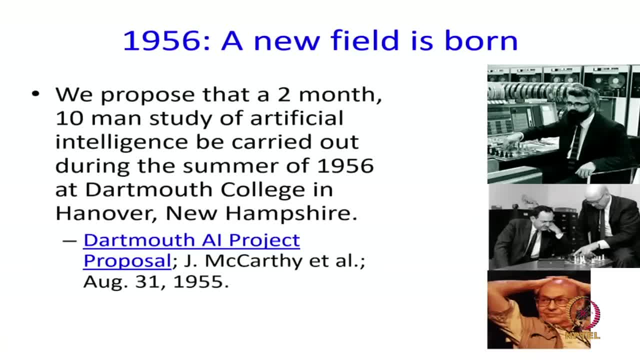 Can we create an AI system which will be able to prove theorems automatically? And lastly, at the bottom, there is Marvin Mintz. He is from MIT who has many contributions, including he built one of the first neural network learning machine. 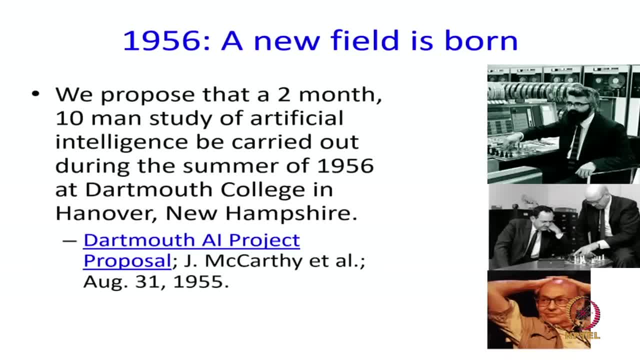 And he is my great great grandfather, at least academic grandfather. So my advisors, advisors, advisors advisor is Marvin Minsky, right, And he was the person who started the MIT AI laboratory. So at the time these four people from Stanford, CMU and MIT came together and officially started 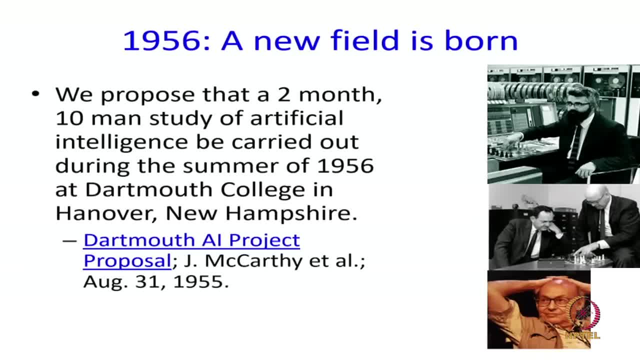 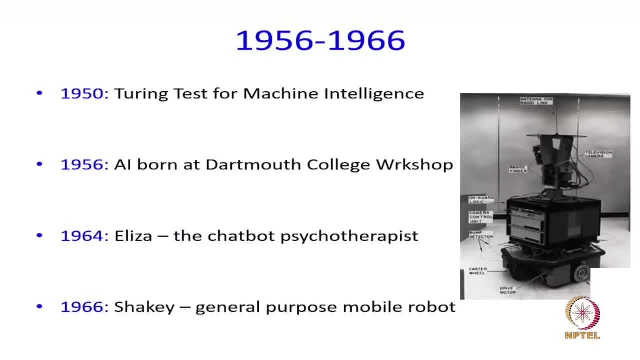 the field. What happened initially? Of course there was enthusiasm, People were coming together and, you know, trying to solve these problems. So if you look at the history, I mean there are many, many things going on, But at the highest level, you know. Turing test came in 50s. AI itself was born in 56,. 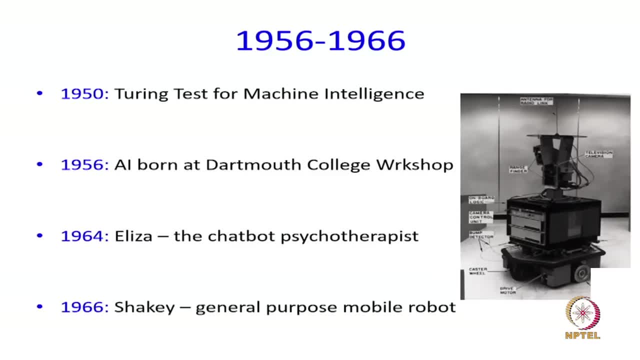 in 64. So, by the way, language and language communication and all that also was part of AI, And Eliza was the first chatbot, way back in 1964,, by the way, we have now. we live in a world where chatbots have become extremely important. 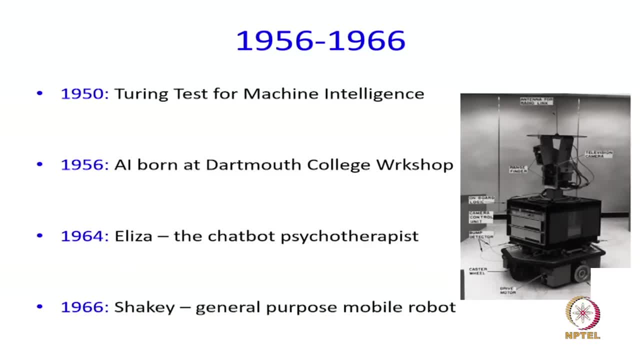 We all have chatbots to play with and you know, spend time with, kill time with, and so on. The first chatbot was in 1964. And, believe it or not, and it is a funny story, where somebody on their private messaging system, instead of having your own response, put Eliza in. 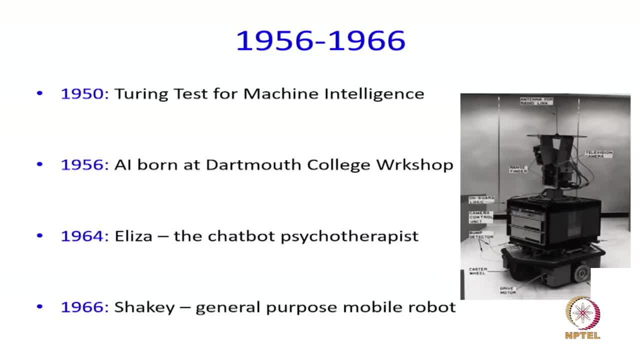 And one person started communicating with Eliza and started getting the Eliza started asking personal questions And this person started answering personal questions. Okay, And this person felt like there was a real psychotherapist sitting on the other side. When we- when you come to my NLP class, we will talk more about Eliza and how to make. 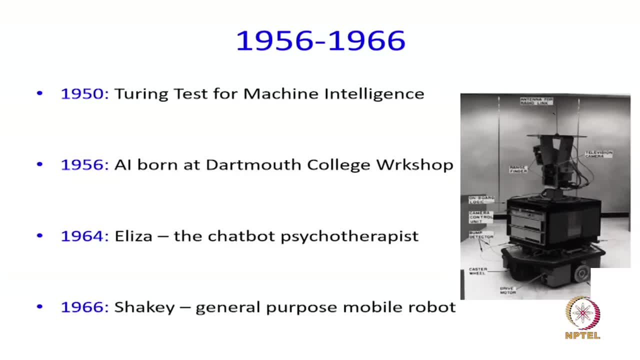 chatbots- not in this course, But this happened way back in the 60s. The first general purpose mobile robot- and you can see a picture on the right- is shaky. you should Google shaky, you should learn about it, and so on. shaky was an amazing project. 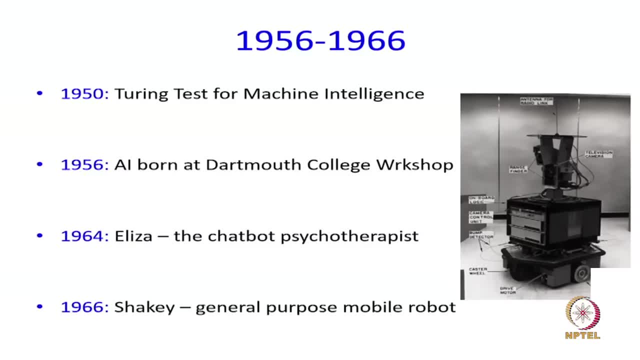 This was this robot which had many, many Sensors and so on. it had a camera control unit, it had a television camera, it had a rangefinder, it had wheels and so on, And at the time people in Stanford were using shaky as a platform to do interesting AI. 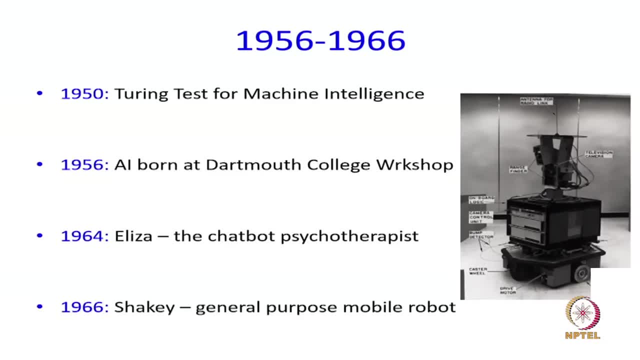 And I remember in 2016, there was a 50 year celebration of shaky at a triple AI conference And a lot of the people who worked on shaky at the time who was still alive. they came together and started narrating very funny stories about shaky and so on. 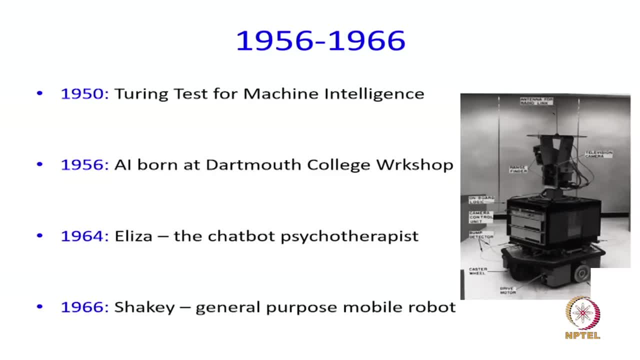 It was really amazing to hear you know. 50 years down the line, shaky was still relevant because in the process they developed one of the most important algorithms of AI called the A star algorithm, And we will talk about A star algorithm and, hopefully, week three. you will see that you 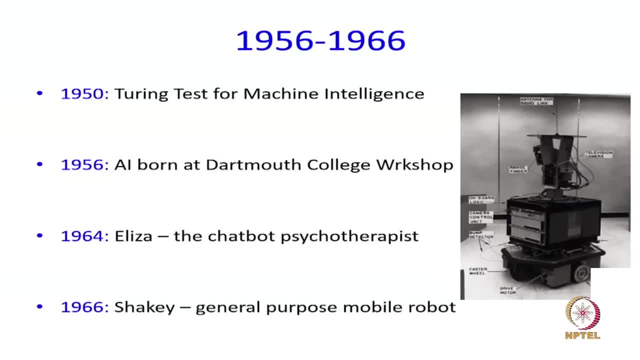 know what happened 50 years ago, 55,, 52 years, 53 years ago was still extremely important and being used in many, many places, including possibly our computer. Okay, Thank you, Bye Bye, Bye, Bye. 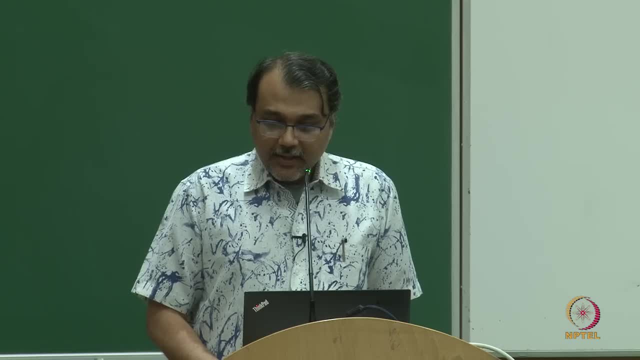 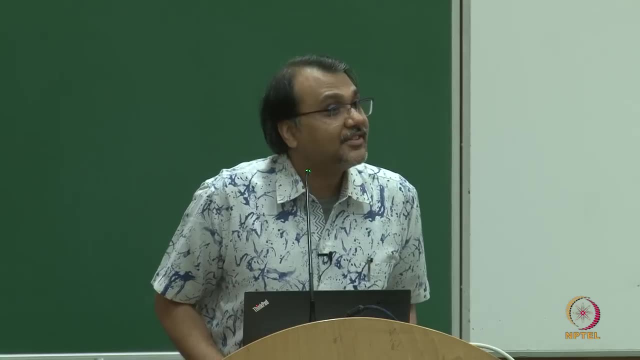 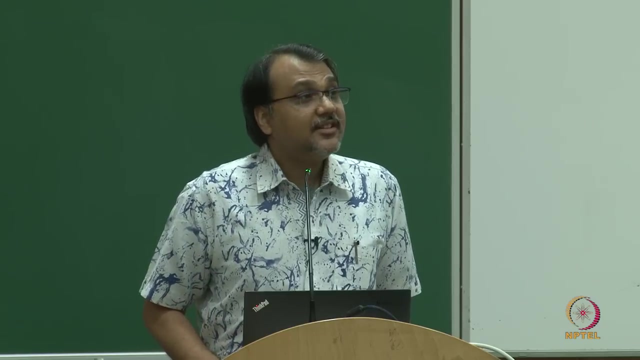 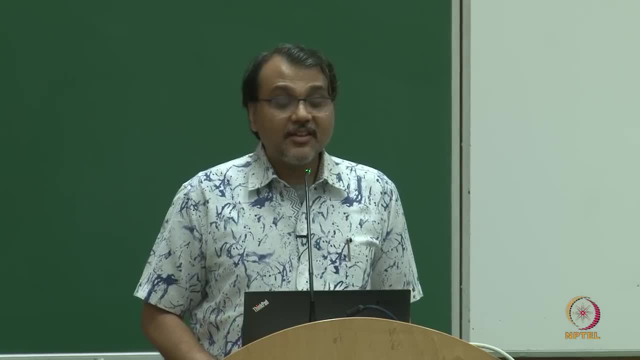 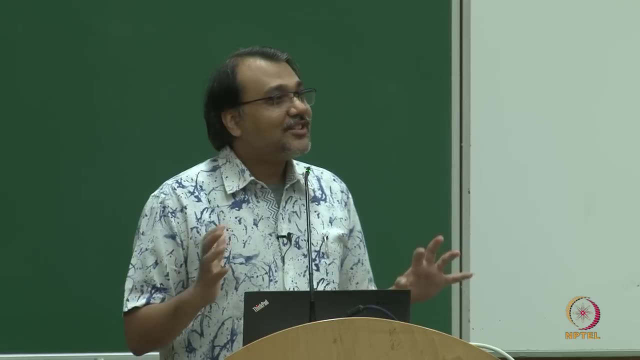 Spring is a great word, but winter is a bad word. So you should think of AI winter not from an Indian point of view where you are like, wow, we have winters now. Wow, You should think of it from a different point of view. 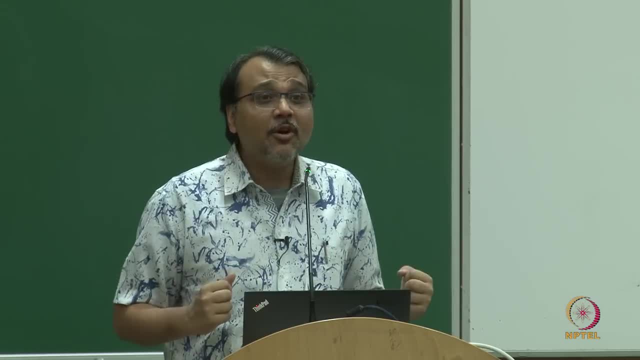 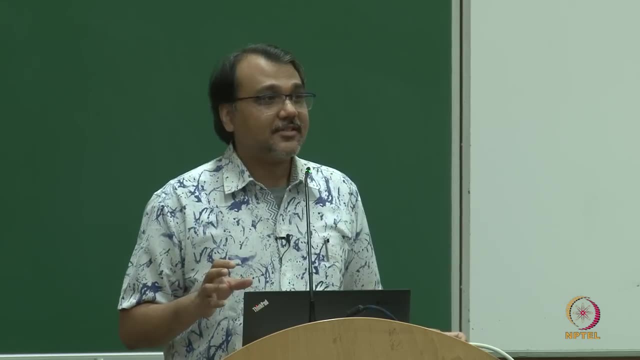 the US point of view, where, oh damn, we have winters. now it is going to snow, it is going to be negative, minus 20 degrees Celsius, or what not. I cannot go out, my eyebrows are going to freeze, and so on, so forth. right, You have seen those videos where you know, put water in the in the air, and you know the. 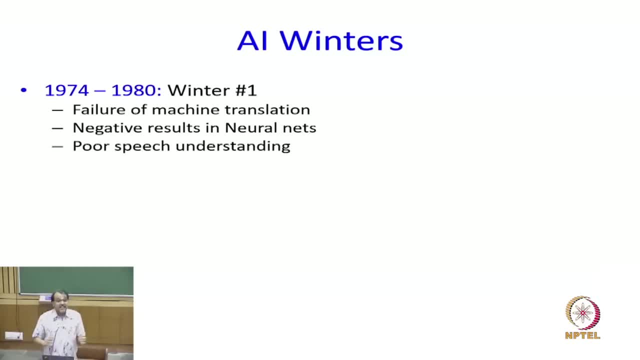 water freezes mid. you are talking about winters and they were winters and they were not one, but there were two AI winters that came over time in 1974 to 80. there was one winter where people who are working in language started to feel that, oh man, this is not working out. 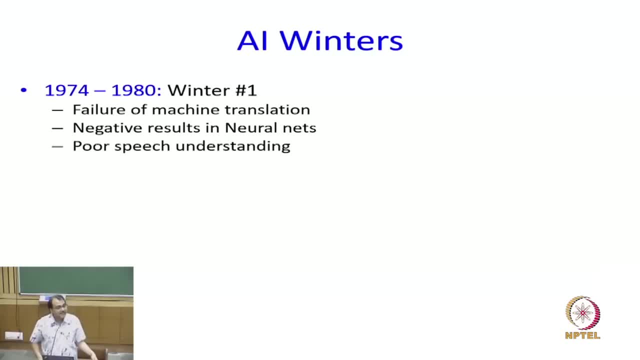 there was one seminal report which said: machine translation is very hard, it is not going to succeed. a lot of funding in machine translation at the time came from defense agencies. can you guess which languages did they care for at the time? English, Russian. we are in the Cold War time. 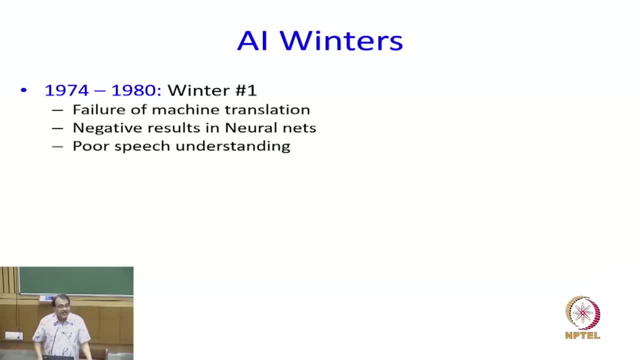 So of course, all the effort was going into making sure that we can understand any things that we can intercept in Russian language. right, and they said that, oh man, machine translation is very hard. Neural network had come in, but Marvin Minsky wrote a paper saying that neural network is. 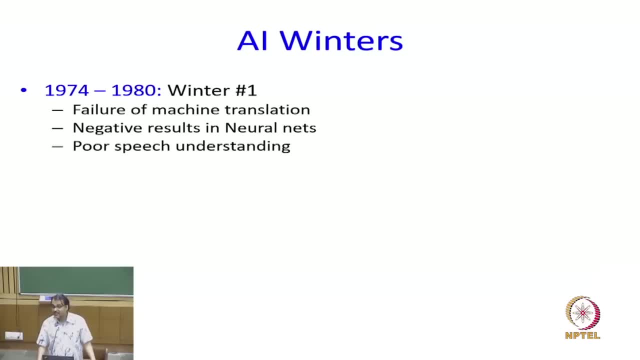 very hard. it cannot even do XOR function. you know XOR function from your logic, I hope. and similarly there was a report. there was some frustration on speech understanding. they were able to show that if you speak words in a certain order, you are able to pass it and 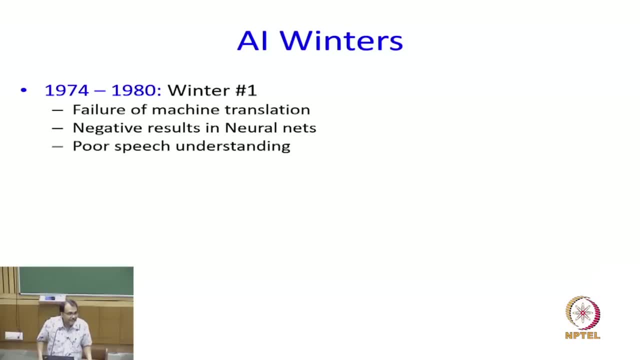 understand it, but otherwise the system can not do anything. and, by the way, all these problems remain unsolved, or mostly unsolved until very recently, and they are still not completely solved, but we have made substantial progress in the last week. So because of all this, suddenly we were in a place where there was so much excitement. 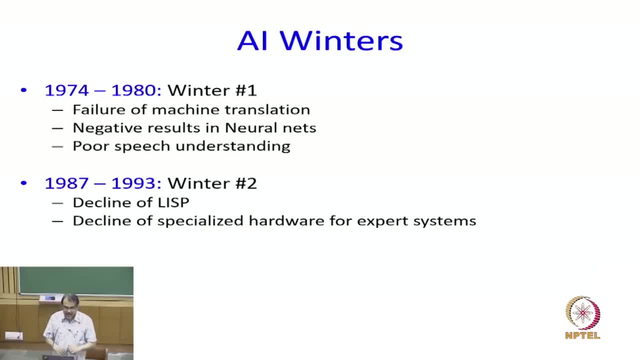 about AI earlier and then it died down. then it started coming back up and LISP was working. there was something called the expert systems error and even now some people who are still stuck in the 90s who teach the old style AI course, they will teach expert systems. 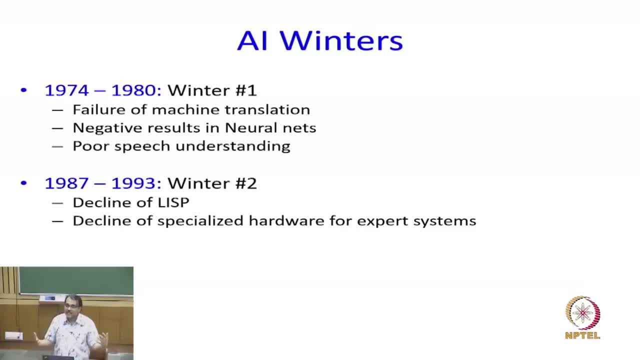 We do not talk about expert systems in this course anymore, because those is this is working from the past. but the idea of expert system was somebody uses a logical language to encode all knowledge about their field. like, if you want to make an automated doctor, you will say that this disease causes these symptoms. this symptom, this disease can be used, can 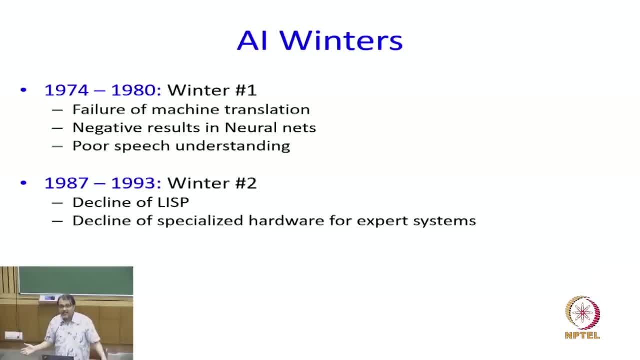 be treated by this medicine, etc. etc. So put everything in a logical framework And then, given the symptoms, you do some inference to figure out what disease you may have, what treatment should be given to you. that was an expert system and at the time they started. 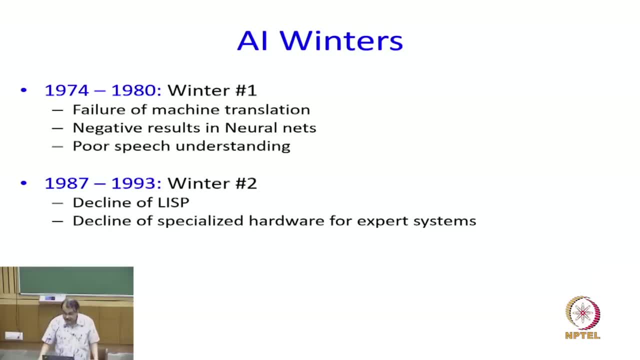 making specialized hardware for expert system and it became a half billion dollar industry. but within a year all that half billion dollar industry was wiped out because new machines came out which which were much better and they were general purpose and so on, so forth, and all this industry died out. 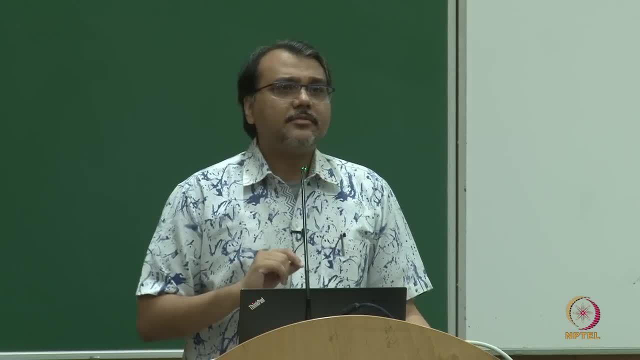 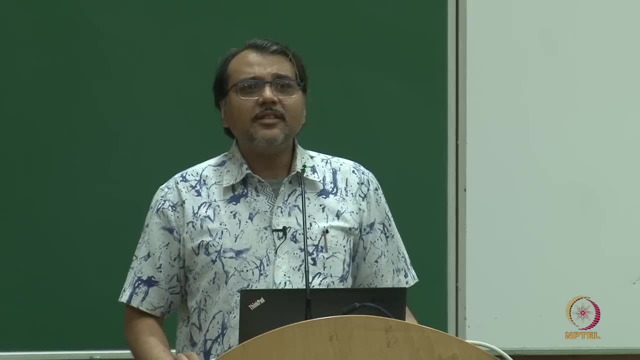 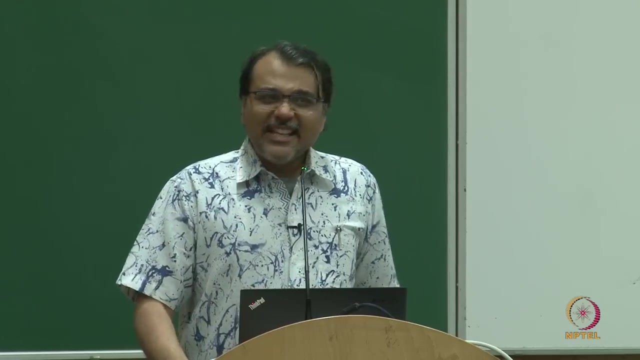 But, more importantly, What died out, what? the reason why AI went through these winters is the because AI researchers were diehard optimists, not cautious optimists or realists. they started saying from the very beginning: we are going to solve intelligence, we will make a machine that will be more intelligence. 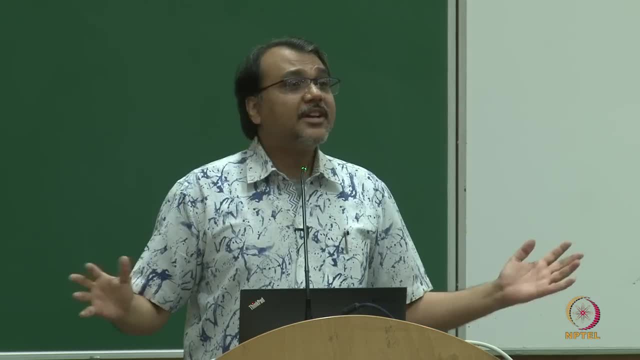 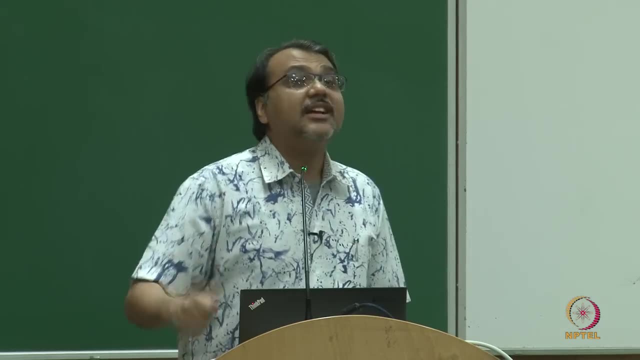 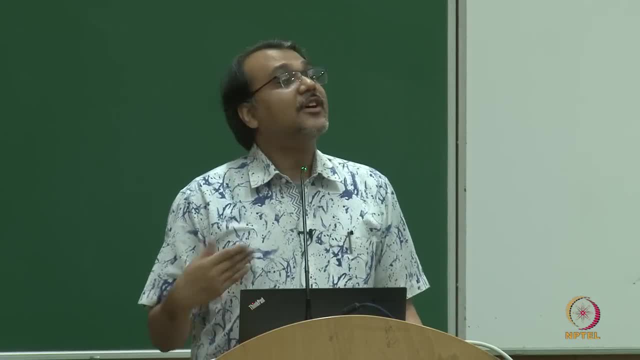 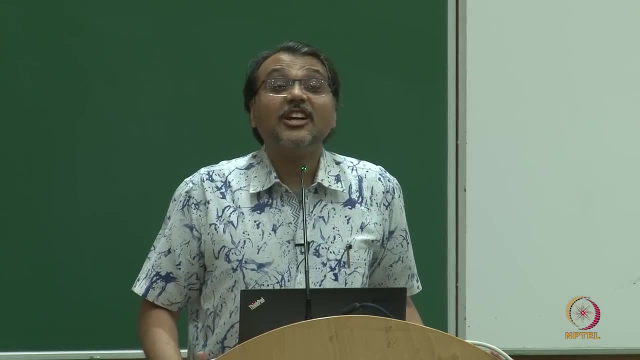 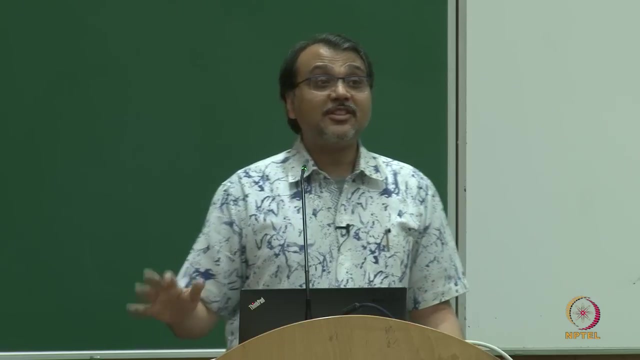 they said, oh, we will give you a million dollars, we will give you 2 million dollars. what happened? what came out? what came out? nothing. I would not sell the money down the drain, but from the perspective of a person who wants to use the technology, they will feel that the money 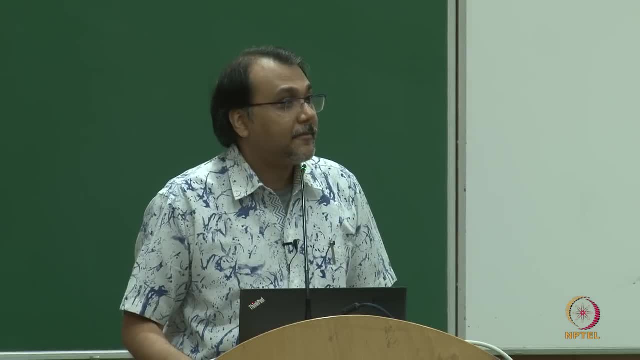 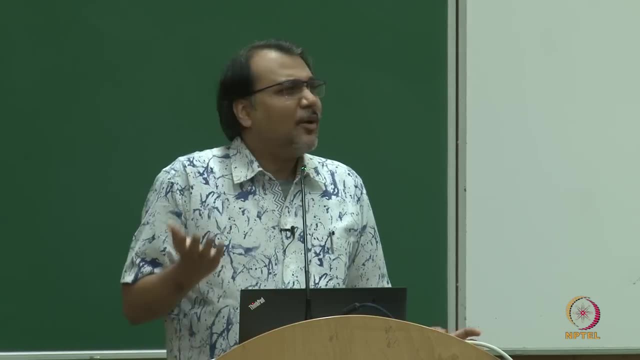 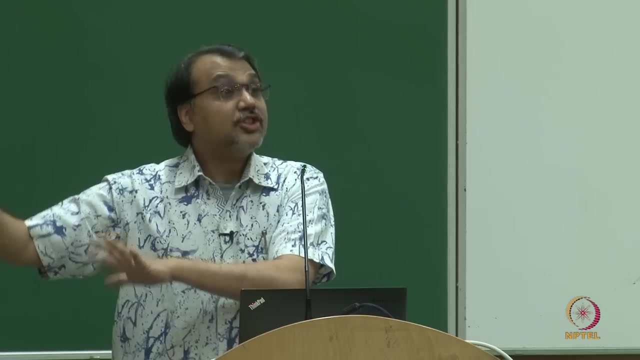 is down the drain because nothing substantial which is workable has come out. So here I started getting bad name to the extent that people thought that Oh, AI folks, these are. the other thing you have to realize is that there were also computer scientists, theoreticians mostly, who really cared about proving things. 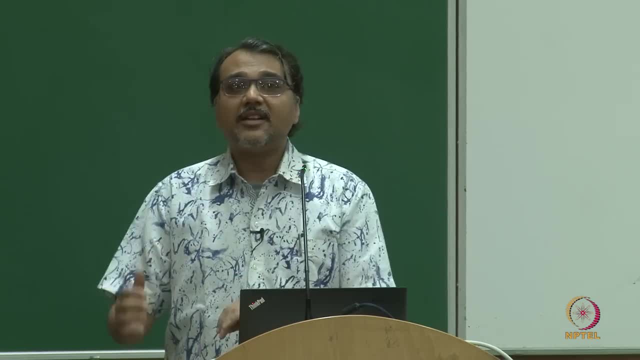 They were like: give me a problem, I will figure out. it is complexity class. give me a problem, I will create an algorithm and prove things about it. On the other hand, is the AI folks was interested in working hard, No matter what. That is what one could do. 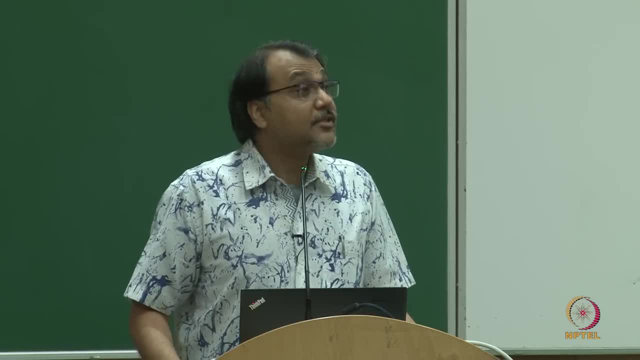 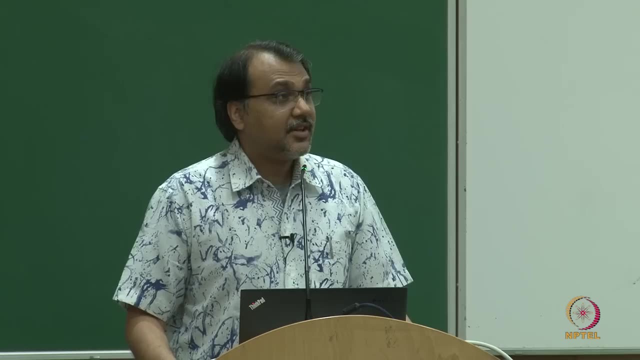 Some may be willing to fix their problems through some kind ofoshop. But what to do? People could do it in working demonstrations. They will prove. but they were interested in working demonstrations more than the proofs, because of which the computer scientist, theoretical computer scientist, 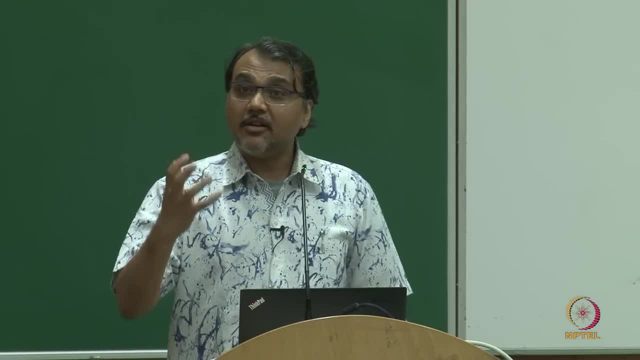 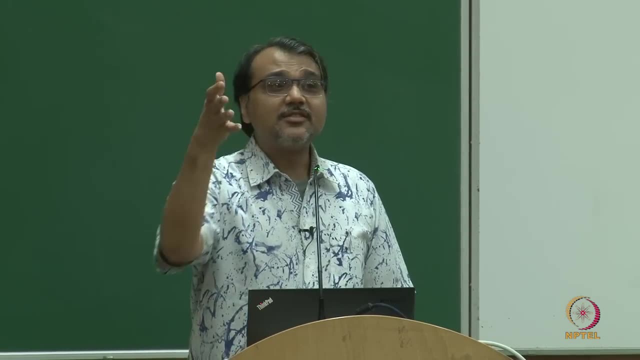 will say: you guys are not formal enough, You guys are not mathematically rigorous enough. On the other hand, the applications people will say: you guys do not. your guys solutions do not work. So they were sandwiched in the middle, neither the applications people are. 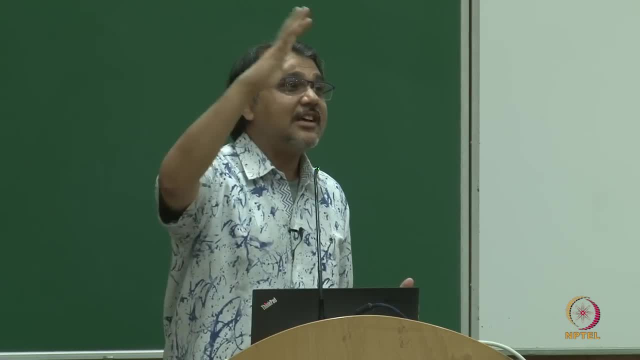 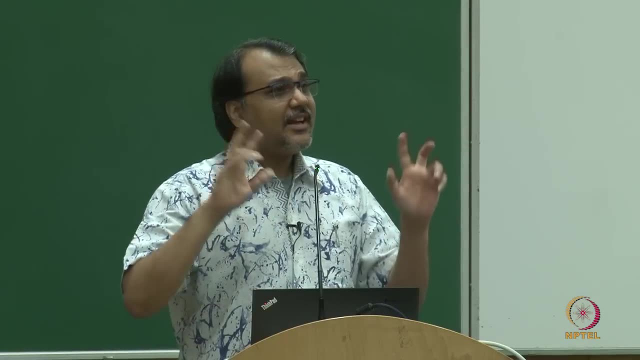 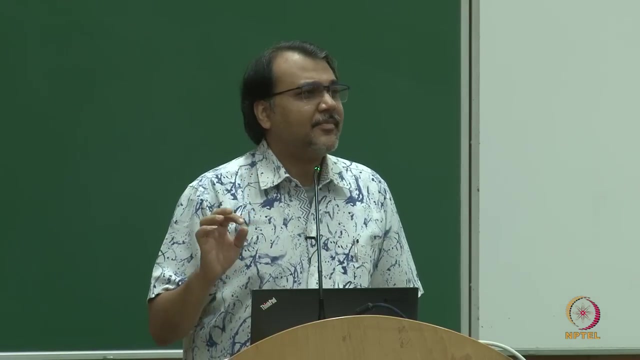 happy that you know you can achieve anything that works. nor the theoreticians are happy. where you can achieve something you can prove anything about. So even in the computer science world, AI started getting bad name. it started being looked at as set of people who have these heuristic techniques, which sometimes work, but have no. 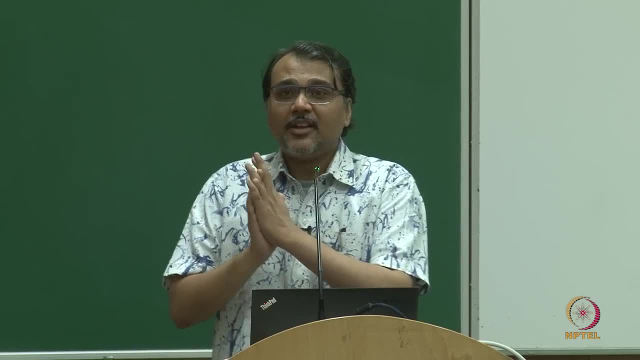 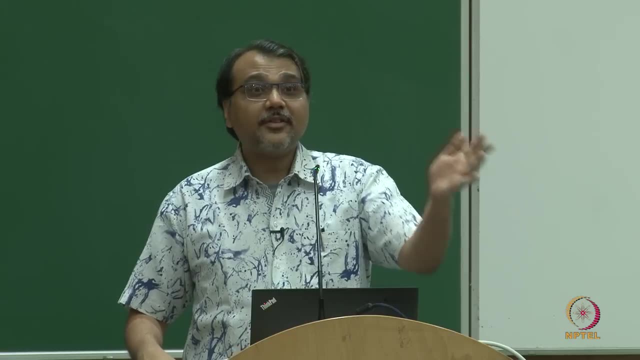 theoretical basis. So, therefore, I remember. and, by the way, some people remain stuck in time, right? You know, for example, after being in IIT for 4 years, if you go home, your mom will still think you are a 17 year old. They would. 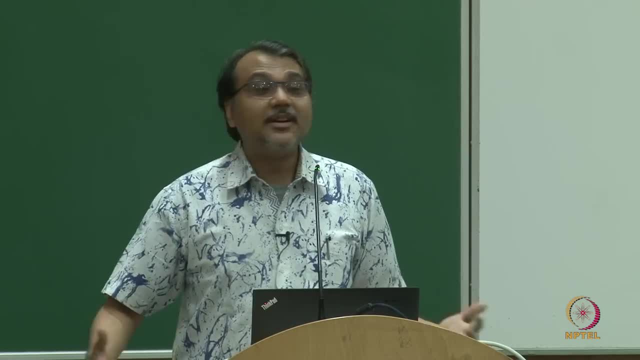 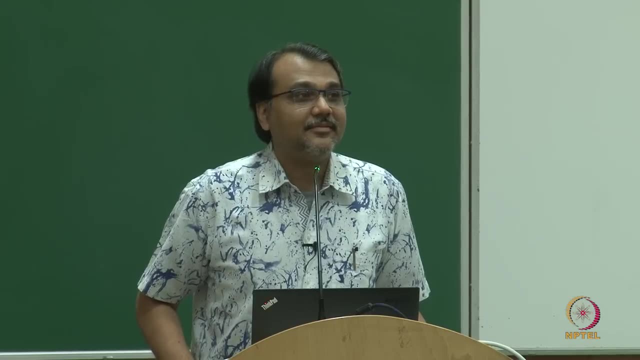 not, she would not know that you are 21 now and you have moved on and you have become a different person. You know, I remember a beautiful talk by Sham Benegal, who said that my mom still thinks I am 14 year old. I am not kidding you. He said that explicitly. We remain stuck in time. 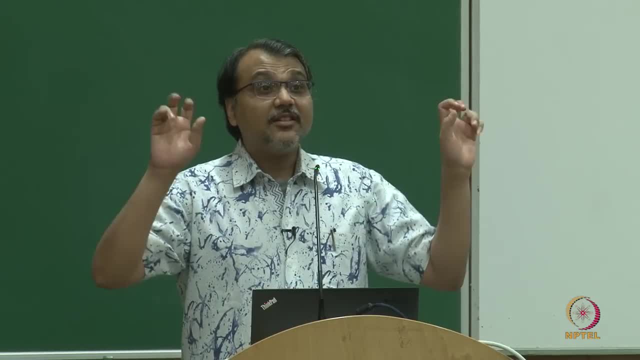 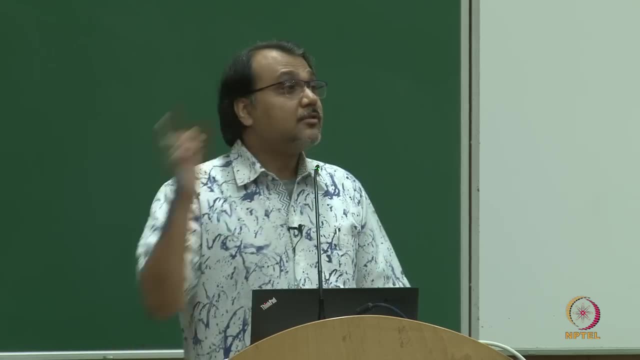 You go to look at your friends who are in the US now, Their notion of India is the notion that was when they left India. So if you look at India, If you go talk to uncles and aunties who left India 30 years ago, their notion of India no. 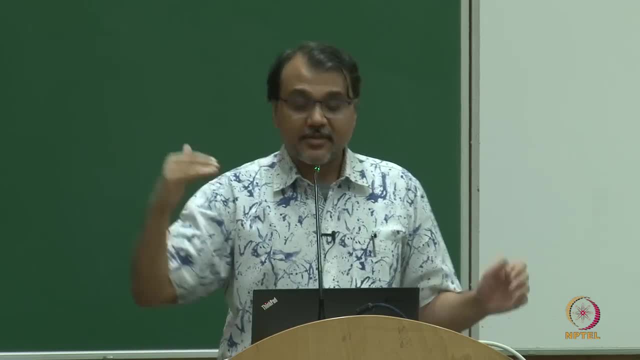 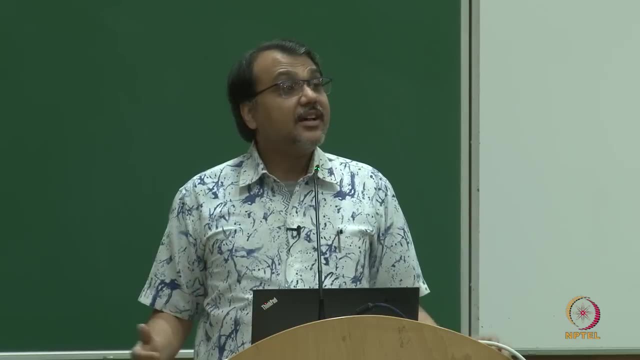 longer matches with any notion of India today, But they are stuck in time, So we are always stuck in time. So they were people, even in this department and in India in general, Who was stuck in time. They thought that AI hasn't moved because they did their PhD in the 90s. 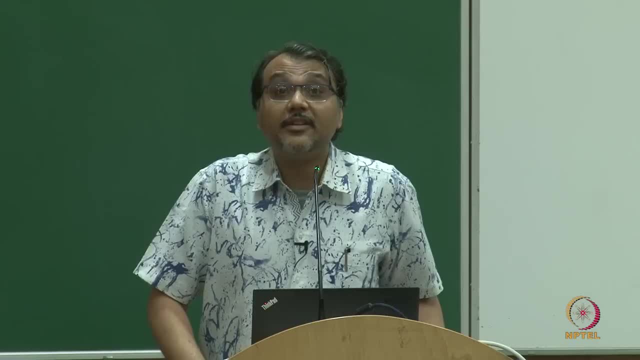 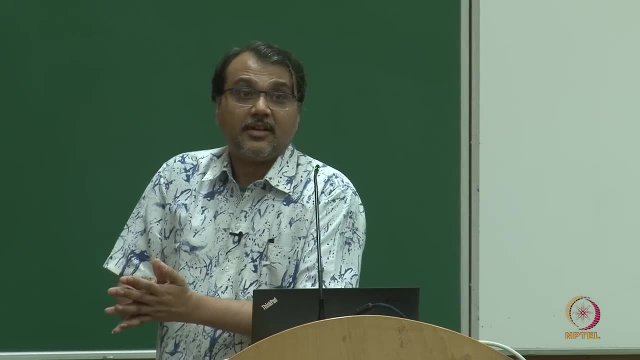 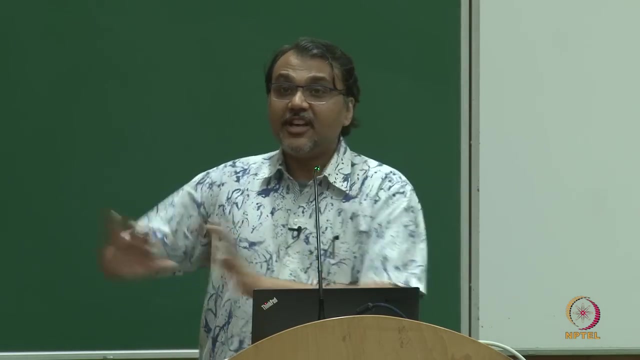 That is where AI was not a very good word, became a bad word. In fact, they were people who cut their cords from AI. They were topics which were part of AI and they created their own sub communities and started saying: we are not AI, we are computer vision. we are not AI, we are natural language. 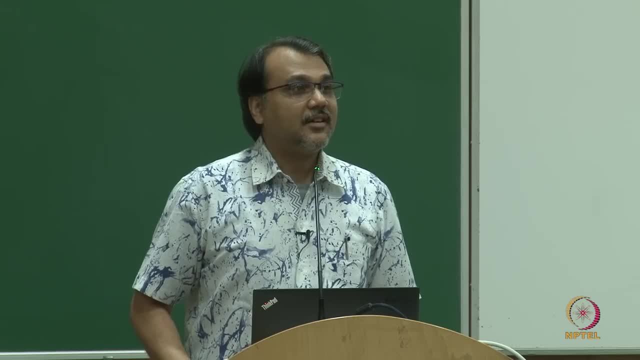 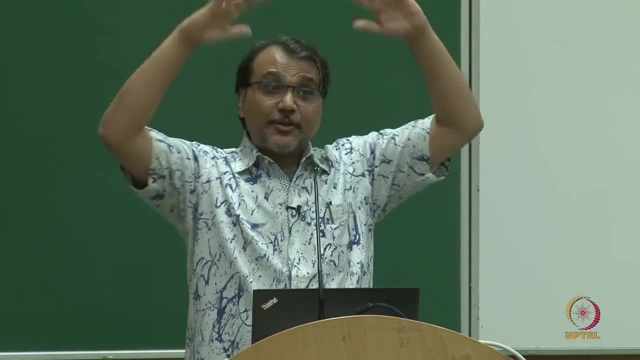 processing. we are not AI, we are machine learning And I lived through that time, therefore I can relate to it. I remember that in 2000s, when I was doing my PhD, triple AI- there were five communities which will still say we are part of triple AI. five is just a number: 3,, 4,, 7, something. 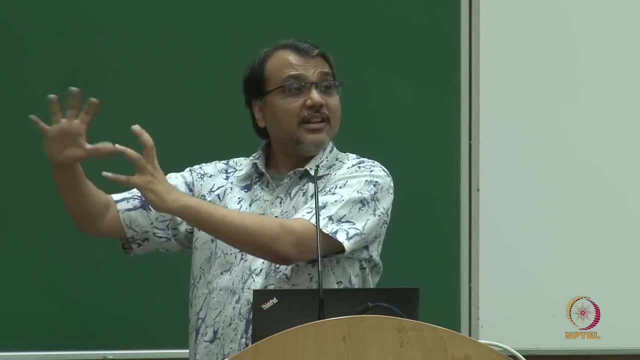 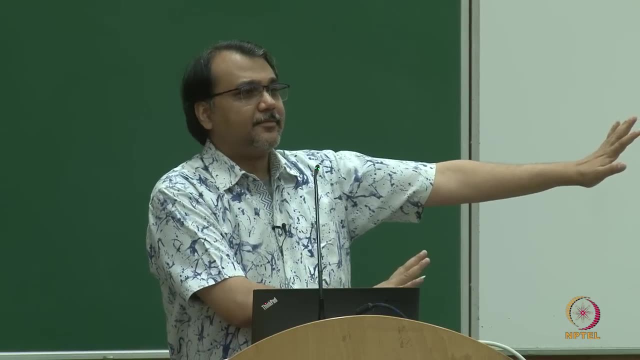 like that, And there were many such communities which will only go to their local conferences when we will never come back to AI conference, Because they thought AI is a bad word. let us stay away from it. Let us say: we are whatever. we are right. 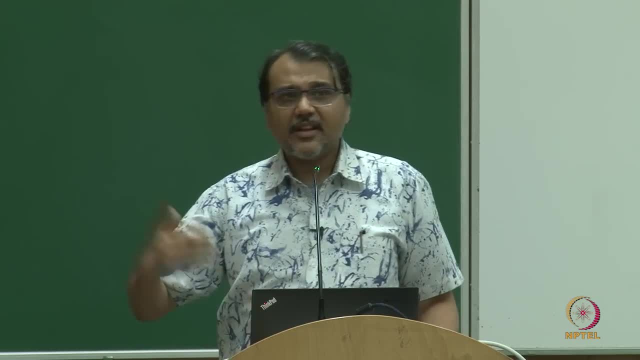 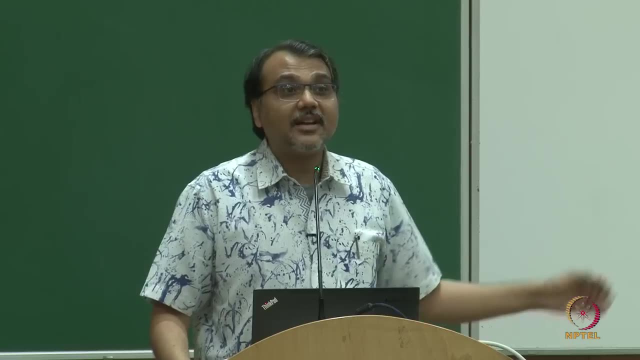 So when I would come back to IIT Delhi, I was a student here undergrad. when I came back as a, I was still doing PhD. at the time I told some of my ex-professors- I mean professors, not ex, they are professors now- my colleagues today- that I am doing AI. they will say: 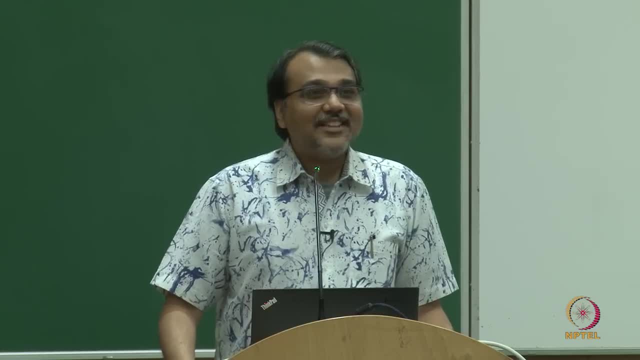 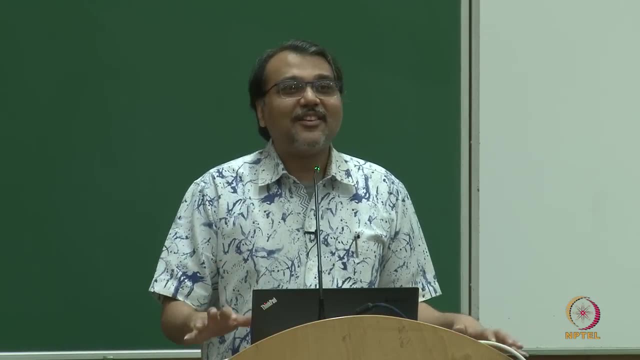 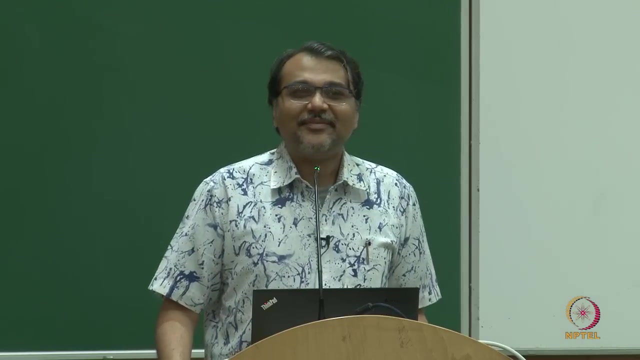 oh, you are doing AI. okay, they will give me the sheepish smile. I do not know why they are giving me a smile, but it was clear that it is not a smile of appreciation. And then I have a one person, who I would not name, who always speaks his mind, thankfully. 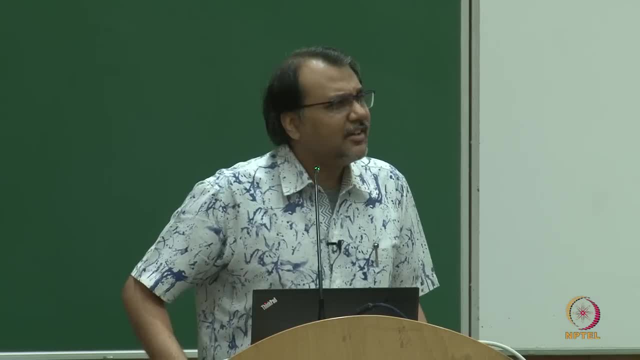 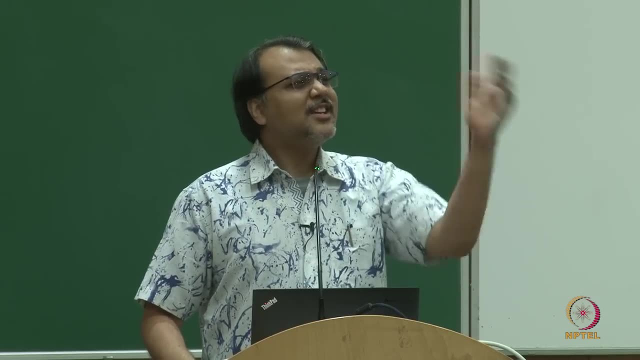 So he said: okay, you are doing AI. what are you doing in AI? So I told him: oh, I am working on this Markov decision process model. oh, so say you are doing operations research. Why do you say you are doing AI? 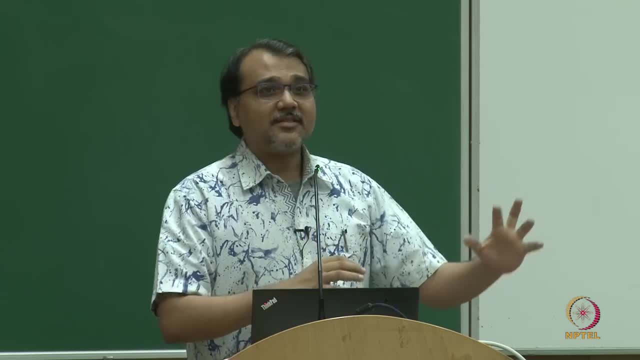 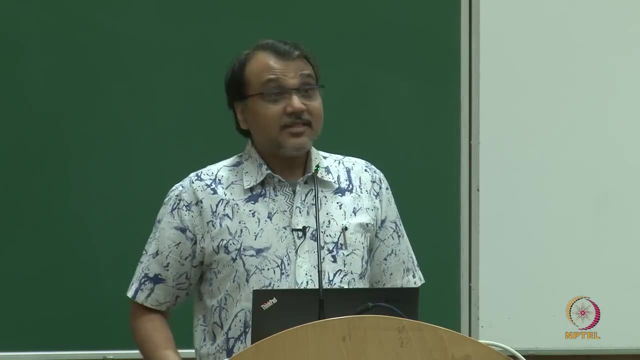 Now for people who do not know, MDPs as a model came from operations research in the 50s. but you know, over time it got adopted by AI and it is the something we will study later in the course. So I was very confused: what is going on? and then it dawned on me that to them AI is still. 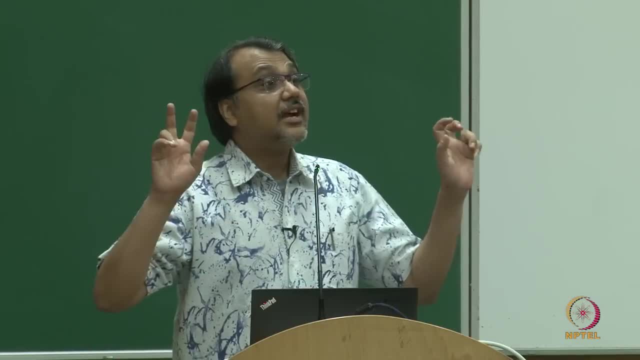 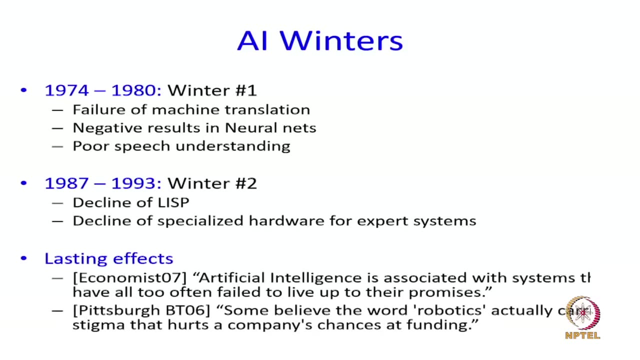 the AI of the 80s and 90s, when we were having AI, winter and AI had become a bad word. So this had lasting effects because- and this is at Economist 2007.. Note, which says AI is associated with systems that have all too often failed to live up to. 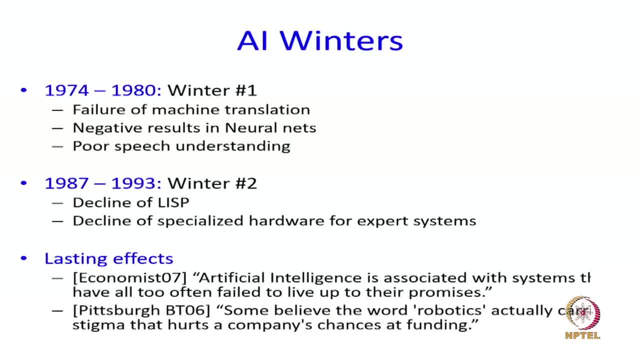 their promises And in this world. over time, AI has now come out and we will talk about the present in the next class, But this graphic shows you the number of attendees for several AI conferences, and at the 80s it was only AAAI and ICHKAI, if you see. 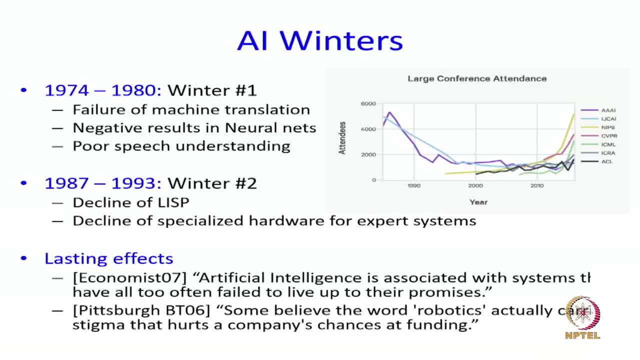 And there were almost 5,000 attendees. So this is the number of attendees for several AI conferences and at the 80s it was only 5,000 attendees. If you see here, there were almost 5,000 attendees at ICHKAI conference in 1985.. 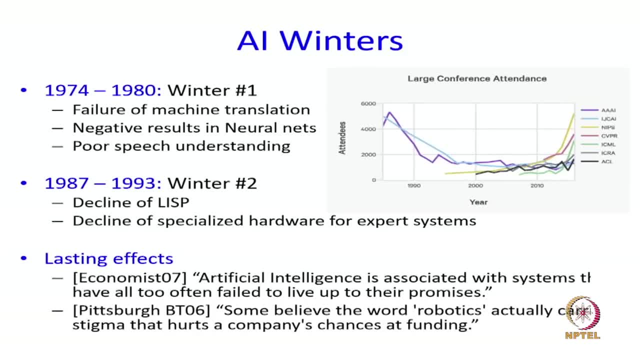 And it went down so rapidly that over time it was less than 2000,. there may be 1500 people started coming. I remember a time when AAAI had less than 1000 attendees And we were very worried that we will maybe even have to close the conference. 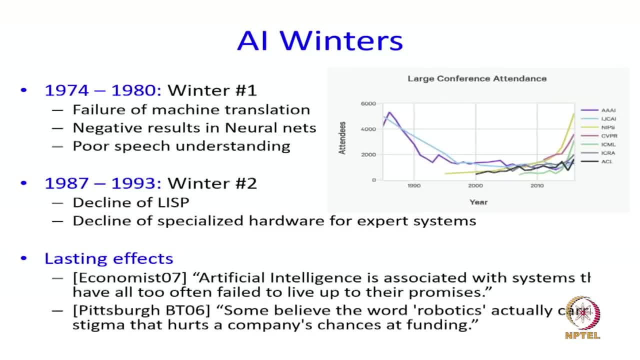 We cannot. we cannot fund it anymore. From there, we have now reached a point where all conferences are starting to see a jump in their attendees And, of course, the conference that has won the most in this is NeurIPS, or NIPS. NIPS is: